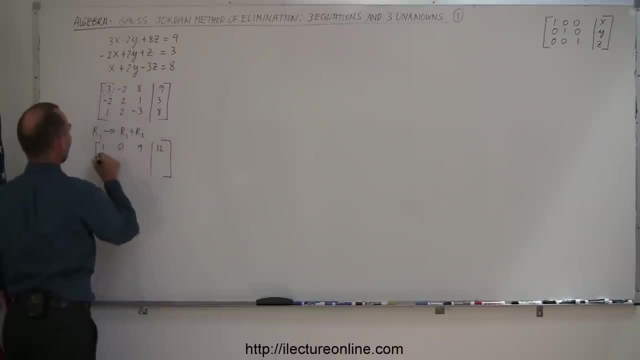 And three plus nine is a 12th, Leaving everything else the same. we have a nine minus two, Two, one, three. we have a one, two negative three eight. I could have also interchanged row one and row three, because if I put this row over there, 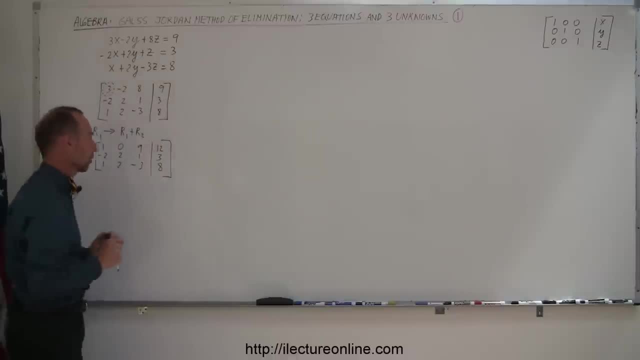 and put this row over there. I would have had a one there as well, So either rule would have worked. Next, we want to get rid of this one and this one, and the way to do that is to take row two- so row two- and replace it by the negative of this number. multiply it times the first. 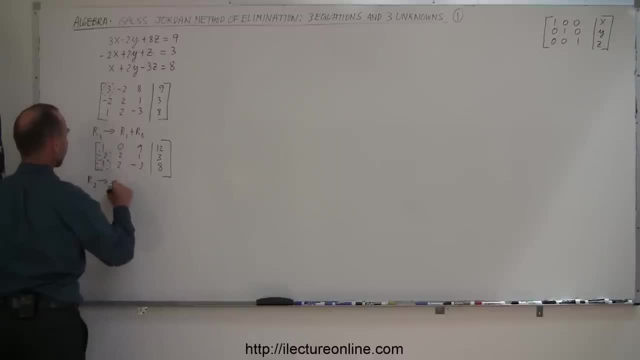 row And add it to this row. So I take the negative of that number, that's two times row one, and add it to row two, And to get rid of this one here we take the negative of this number. so row three is replaced. 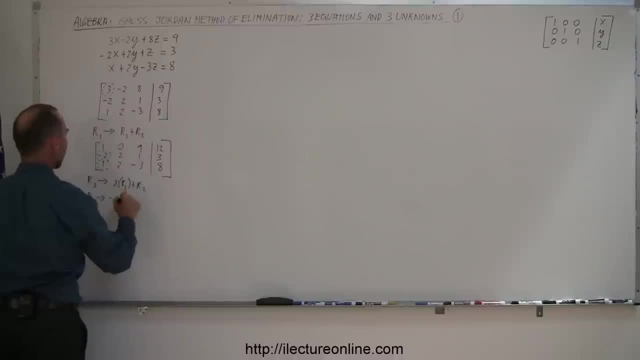 by the negative of this number, which is negative one times the row with the one in it, and adding it to row three. So we're going to do those two steps together. So then I end up with the following result If I take two times row one. 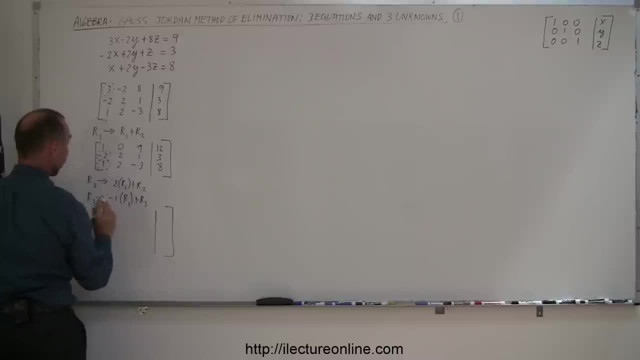 Two times one and add it to negative two, I get zero. So or, by the way, let me put row one down first, because I'm not going to change row one at all. I'm only changing row two and row three. 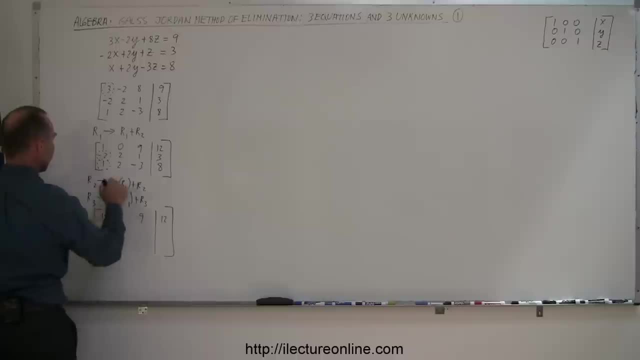 So, two times one, add it to this, gives me zero. Two times zero, add it to two, gives me two. Two times nine: 18, add it to one gives me 19.. Two times 12,, 24, plus three gives me 27.. 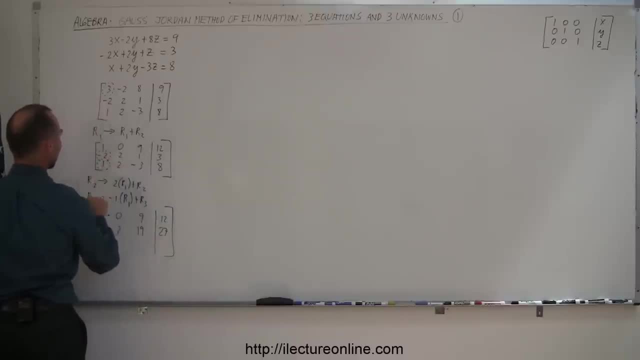 And for the third row, I'm going to take negative one times this. add it to row three. So negative one times this. add it to that. That gives me zero. Negative one times this, add it to two gives me two. 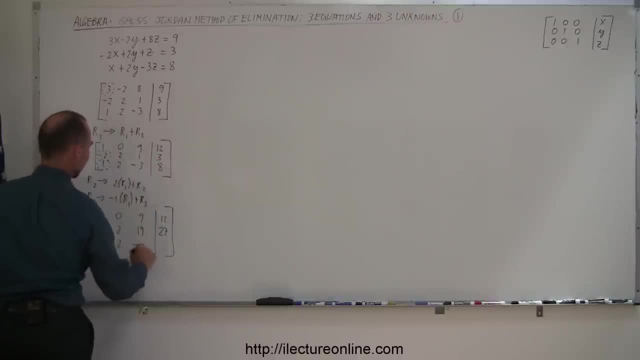 Negative one times nine is negative nine. add it to negative three is minus 12.. And negative one times 12 is negative 12, add it to eight gives me negative four. So now I've gotten a zero here and a zero there. 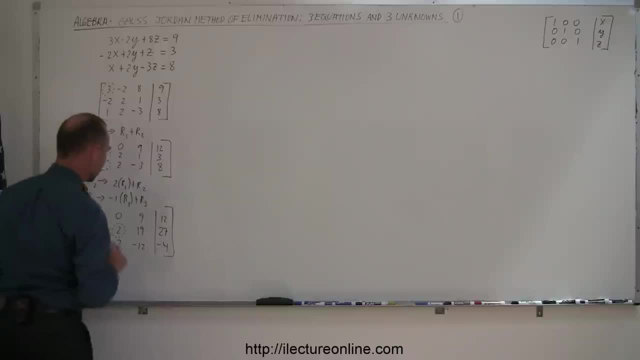 Next, I'm going to attack this one. I want to turn that into a one. The way to do that would be to take the whole row and simply divide it by two. So I'm going to do that. So take row two. 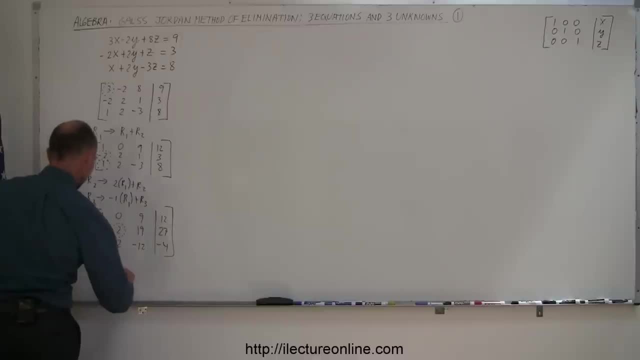 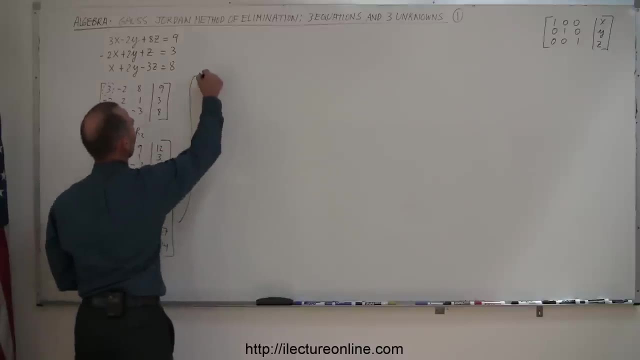 Take row two and replace it by one half of row two. So what I'm saying here is simply divide row two by two. If I do that, I get the following matrix: What is not changing? Of course, row one and row three are not changing. 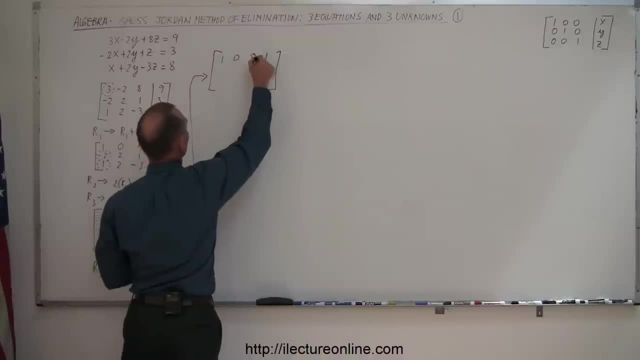 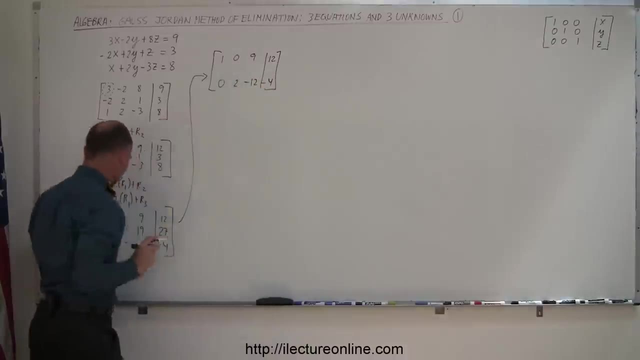 So I get a zero, a one, a zero a nine and a 12.. And I have a zero, a two, a negative 12, and a negative four. So row one and row three are not changing Row two. 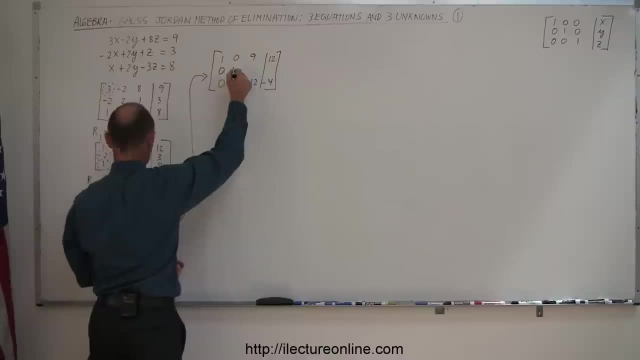 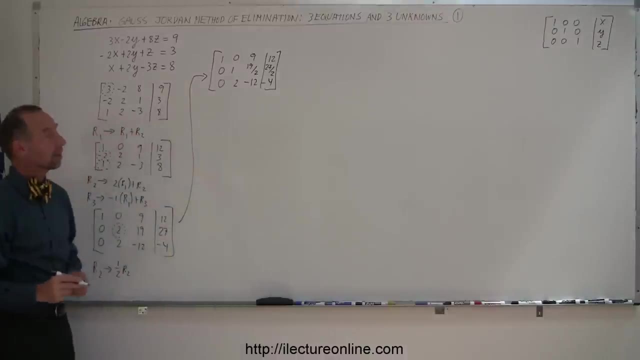 I can do half of what I had there before. So this becomes zero: one, 19 divided by two and 27 divided by two. All right, Now the next step is to turn this and this into zero. Since that's already zero, I only have to worry about this one right here. 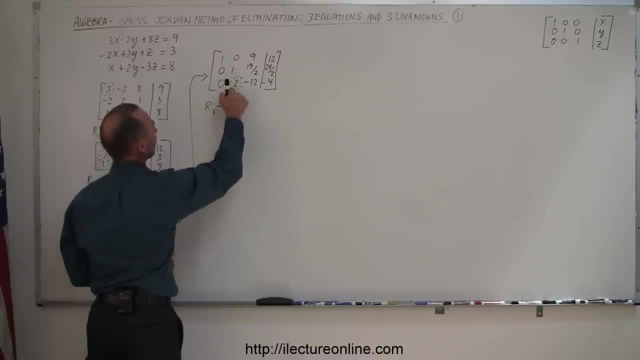 So I'm going to take row three and replace it by the negative of this number, times the row with the one in it, which would now be row two, and adding it to row three, And by doing that, this should go to zero. 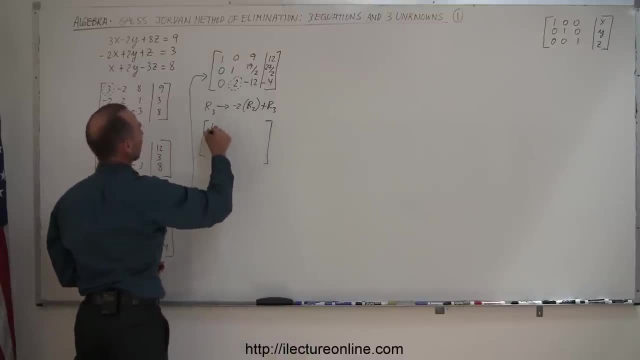 Let's see what happens. So I'm not changing row one at all, so that's still a one zero nine and 12.. I'm not changing row two, so that's zero one, 19 over two and 27 over two. 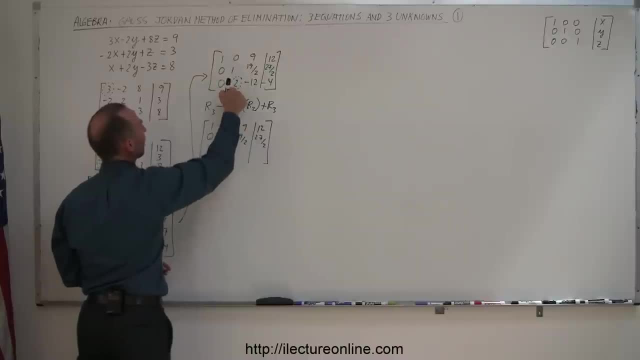 But I'm changing row three. I'm taking negative two times this and adding it to this. So negative two times one. adding it to two, it gives me zero. This is, of course, still zero. That's zero. Negative two times this gives me minus 19.. 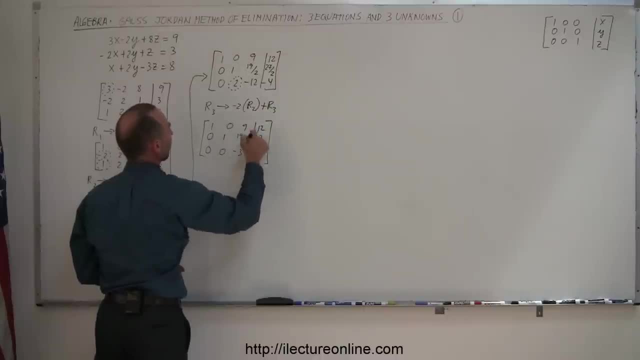 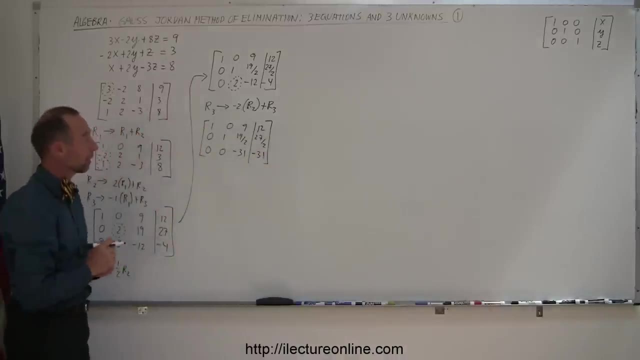 Add it to minus 12.. That gives me minus 31.. Negative two times: this gives me minus 27.. Add it to negative four, It gives me minus 31.. All right, I'm getting closer now. I already have the first two columns looking the way I want to. 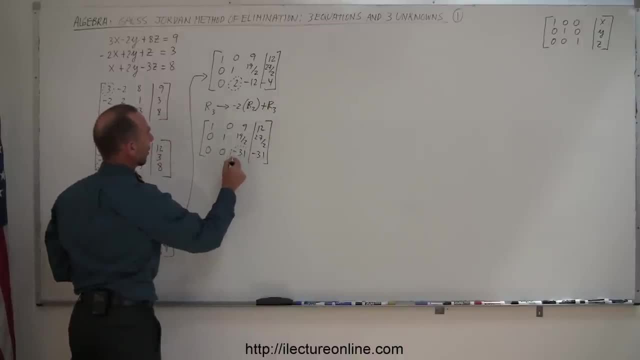 Now we go to the third column. I start with taking this number right here and I want to turn that into a one. To do that, I have to divide this by a negative 31.. So row three becomes row three Divide by a negative 31.. 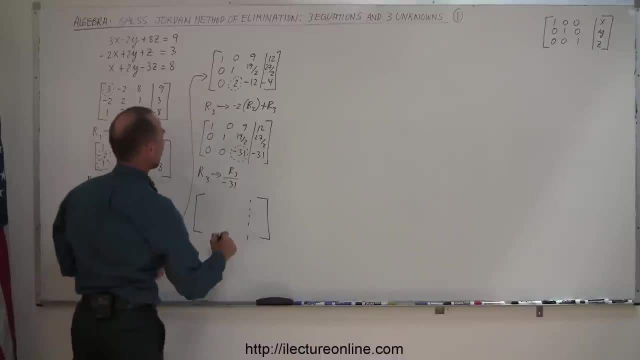 Okay, If I do that, the other two rows stay the same. So this becomes a one, a zero, a nine and a 12. Zero one: 19 over two and 27 over two. Next, I'm going to turn this one into something that will give me a one there. 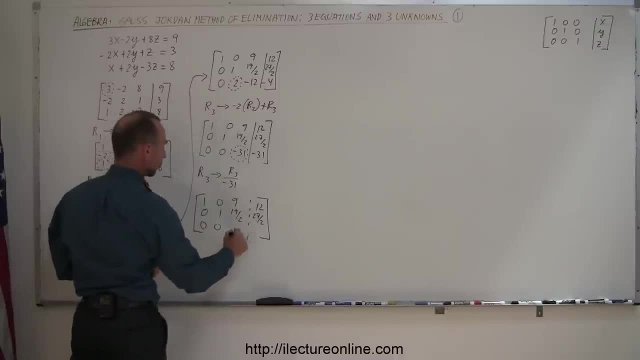 So that's zero, zero. This, divided by a negative 31, is, of course, a one. This, divided by a negative 31, is a one. Okay, Very good. Next, I want to take this, I'm going to take this and turn those into zeros. 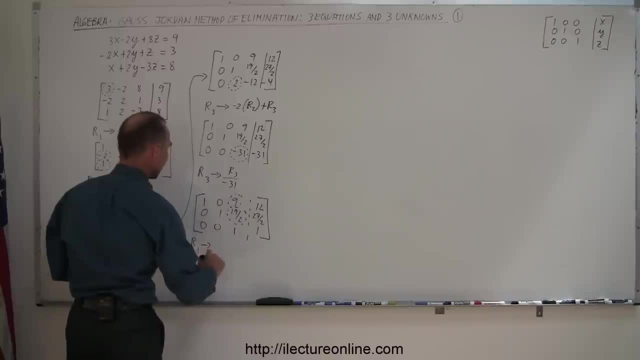 To turn the first one into a zero, R1, I'm going to replace it by the negative of this number minus nine times the row, with the one in it which is R3, and maybe I should make this a solid line, so it's a little better to see- and then adding it to row one. 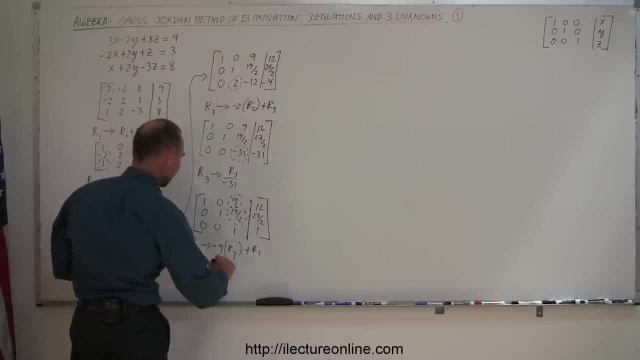 Take row two. I take the negative of this number, so minus 19 over two. multiply it times row three and adding it to row two. By doing that, those two numbers should go to zero. So let's see what happens. 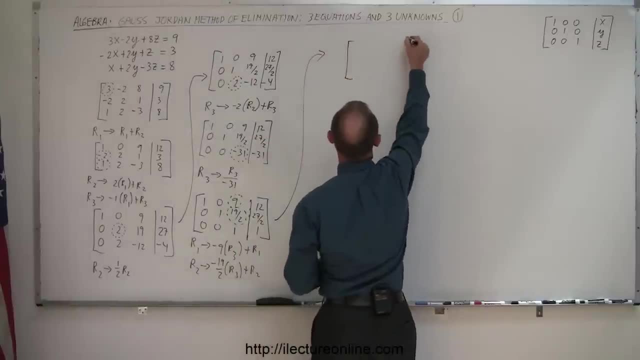 Coming over here. What is not changing here? I'm not changing row three. Row three stays the same, so zero, zero one and one like so. So for row one I take minus nine times this. So minus nine times one is minus nine. 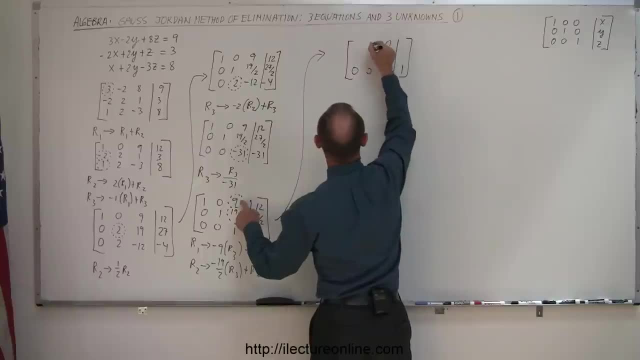 Add it to nine, I get zero. And of course I still have the one and the zero there. That doesn't change. So minus nine times one. adding it to 12, that gives me three. Okay, Row two: I take minus 19 over two times this. adding it to that, that makes zero. 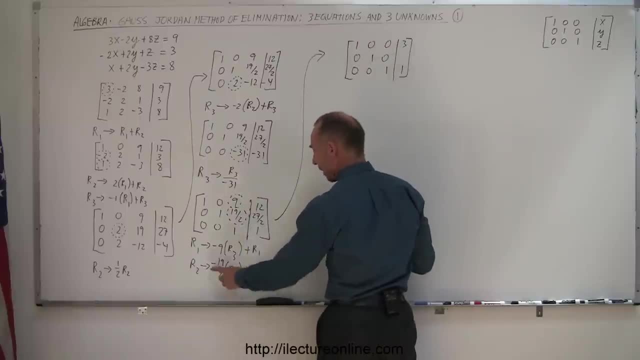 So I get zero, one zero And minus 19 over two times this. add it to 27 over two, so minus 19,. add it to 27,. that gives me plus eight over two, and eight over two is a four. 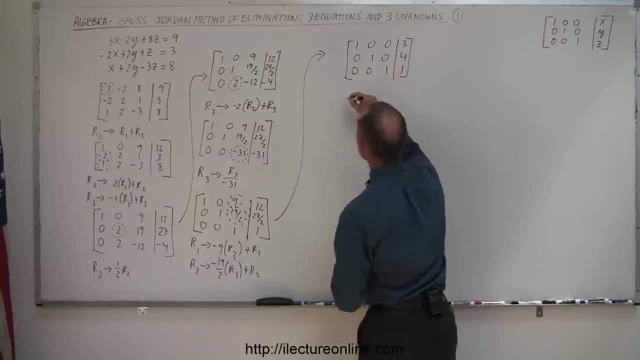 And I'm done. I have exactly the format I want here, Okay? Which means one times x is three, so x equals three. One times y is four, so that means y equals four. And one times z is one, so z equals one.